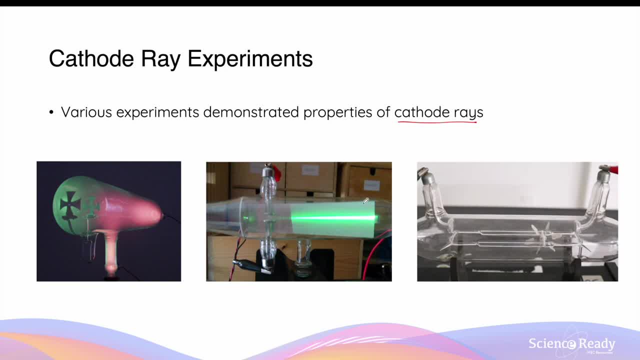 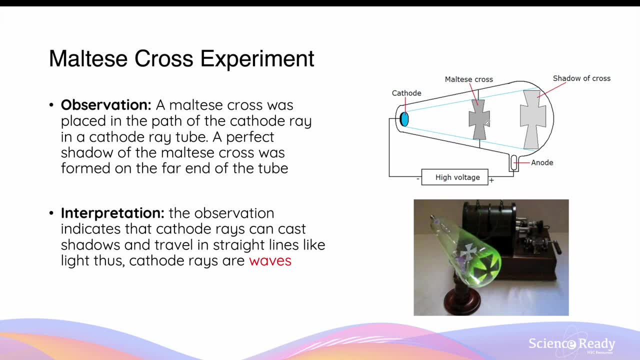 properties of the cathode ray. We'll go through each of these experiments and discuss what exact property they demonstrate. The first experiment involves placing a Maltese cross metal plate in the path of the cathode ray, between the cathode which emits the cathode ray and the anode, which is positively charged. 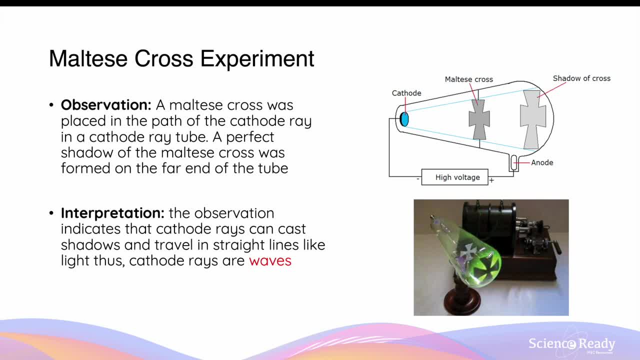 When the Maltese cross is present, a clear shadow in the shape of a Maltese cross is casted directly behind the Maltese cross. This is the green fluorescent light that is normally formed behind the anode in the cathode ray tube. This observation indicates that cathode rays can cast shadows and travel in. 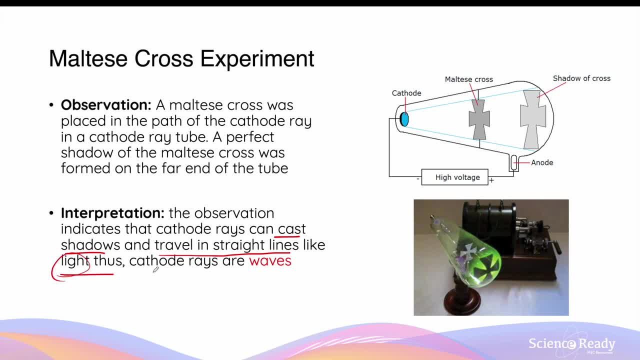 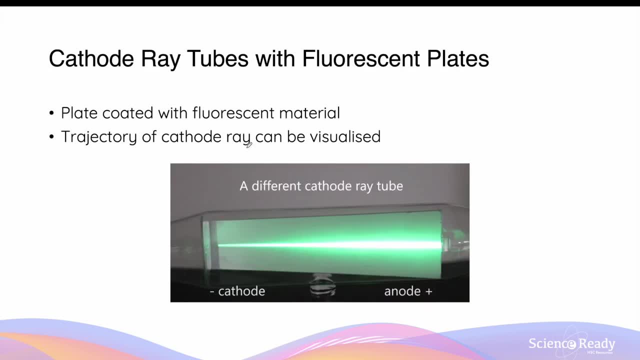 a straight line, just like light. Since light is a wave, they hypothesise that cathode rays are also a wave in nature. Experiments using cathode rays were also conducted using fluorescent plates. In the cathode ray tube, a long plate is coated with a fluorescent material to help. 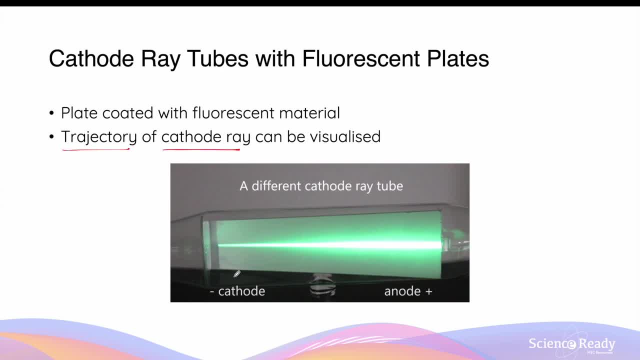 us visualise the trajectory of the cathode ray. In this diagram, the cathode ray is produced from the cathode, which is negative, and travels towards the anode, which is positive. This can be visualised by the green streak of fluorescence that is enabled by placing the metal plate that is coated with a fluorescent material. 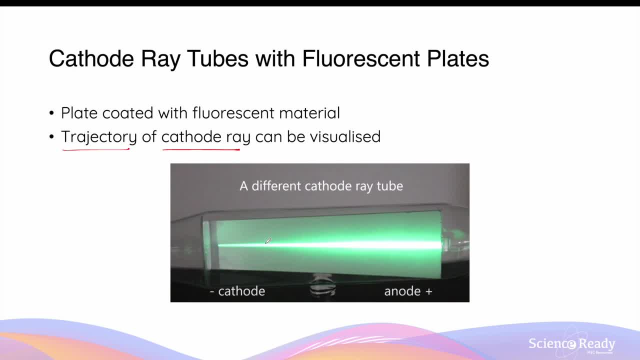 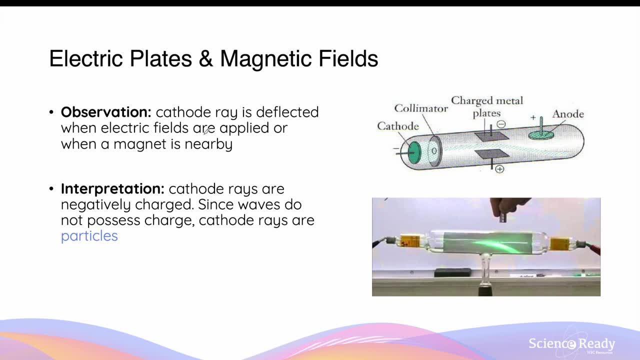 in the background. Normally, the cathode ray will travel in a straight line directly from the cathode to the anode. Experiments using the fluorescent plates were investigated using the helemaal plates and magnetic fields. They observed that the cathode ray is deflected. 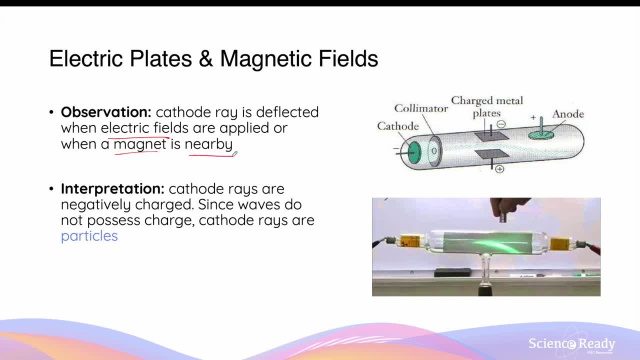 when the electric fields are applied or placed nearby. In the diagram, two charged plates are placed at the top and bottom of the cathode ray tube, being positive, And the cathode ray trajectory is deflected towards the positive plate. In the bottom diagram, a permanant magnet is placed nearby the cathode ray. As a result, 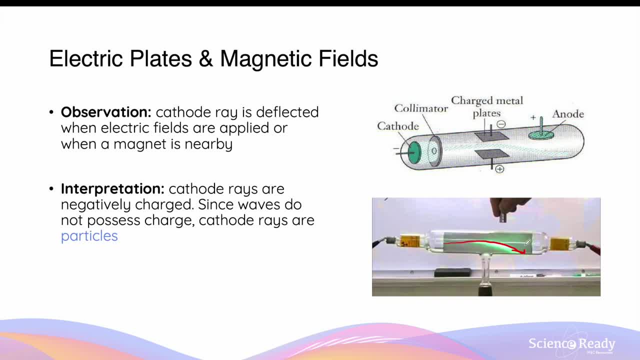 the trajectory is perfect, but the path of the cathode ray trajectory is not perfect, so why do we think it is perfect? There are two провums that are connected to each other of the catheter ray is also deflected towards the bottom. The deflection of the catheter ray. 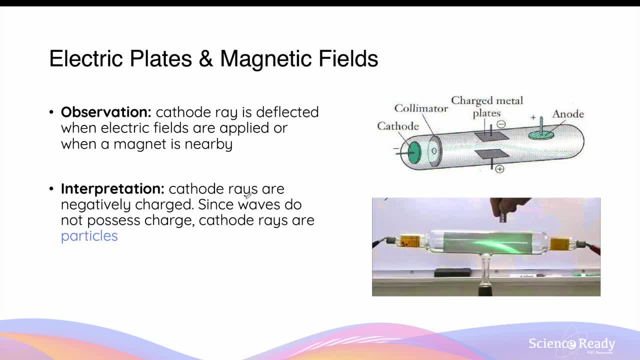 in the presence of electric fields and magnetic fields suggests that the catheter rays are charged, specifically negatively charged, because they are deflected towards the positively charged metal plates. Since waves do not possess charge, these experiments support the idea that catheter rays are actually particles in nature. Another famous experiment involving catheter ray tubes.